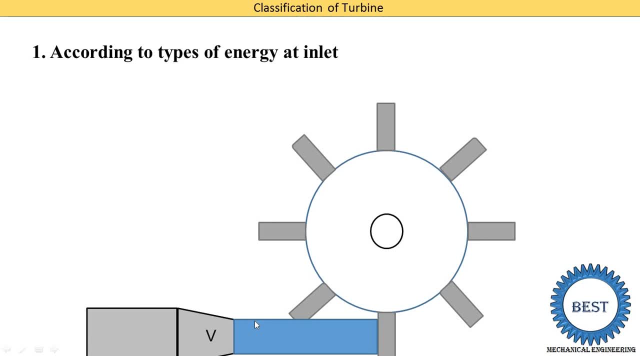 energy, kinetic potentials and pressure energy. So according to this type of energy, the turbine is divided into two categories. First one is the impulse, Second one is the reaction turbine. So first one is the impulse turbine. Impulse turbine means at the inlet of 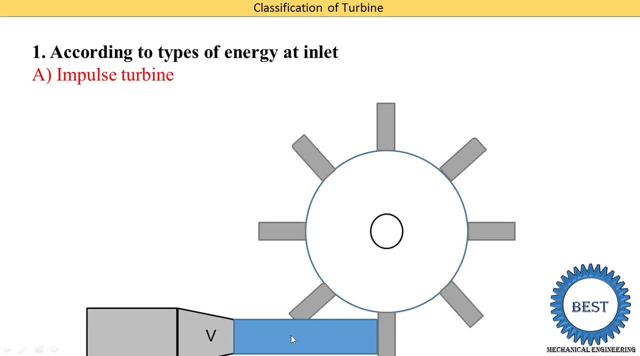 the turbine. this is a turbine, and this is the blue color is the water. So this water have a only kinetic energy. That means pressure. energy is atmospheric pressure, So this is known as the impulse turbine. So again, I repeat, at the inlet of the turbine, this is the water. So 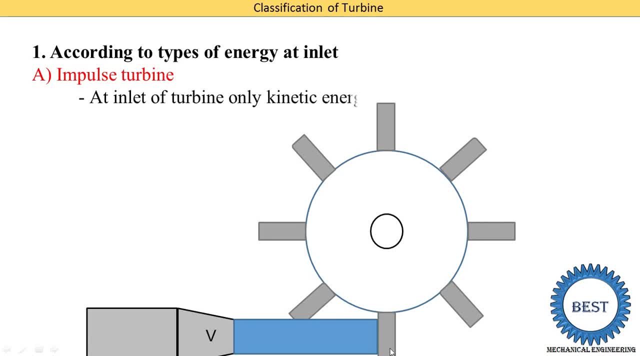 this is the impulse turbine. Now the majority is a three types of the turbine, three types of turbine. that is, a Pelton, Francis and Kaplan. Now, out of these three, Pelton wheel turbine is examples of an impulse turbine. So that is only one turbine. it is a impulse turbine. 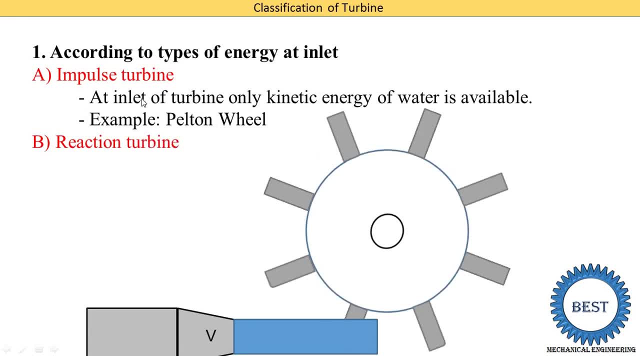 and it is known as the Pelton wheel turbines. So these classifications are most important on the basis of different government exams. that they are always asking one or two questions from this turbine or a one table is asking to make the right tables now. second, is reaction turbine in a reaction turbine at this inlet. 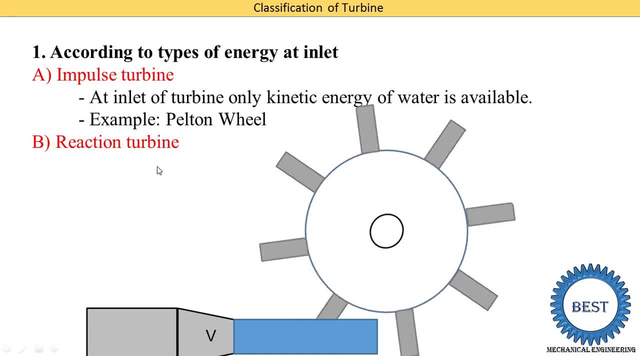 of the turbine, the water, have a two types of energy. one is kinetic energy and second one is the pressure energy. so at the inlet of the turbine kinetic as well as pressure energy of the water is available, means pressure at the inlet of a turbine is greater than. 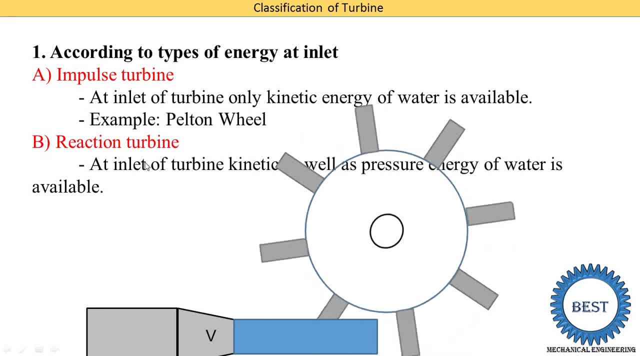 at at atmospheric pressure and velocity is also high. so it is known as the reaction turbine. in reaction turbine, that is a two examples. first one is the Francis turbine and second one is the Kaplan turbine. so Francis as well as Kaplan, both are the reaction turbines, and in impulse turbine that is only one. that is a Pelton wheel turbine. now the at the last. 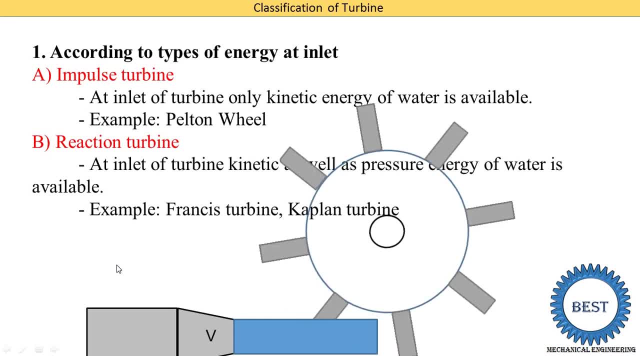 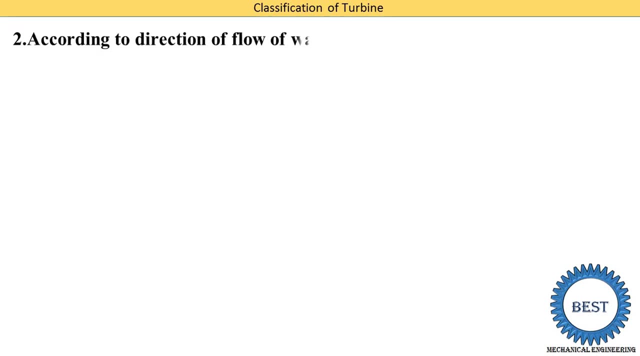 of the video. I give you the trick of How to remembers the complete classifications. so, and up to the last, before that, i request to subscribe my channels and like the video now. second is according to the direction of water supply to the runner. so, on the basis of, there is a four type of the flow. one is tangential. 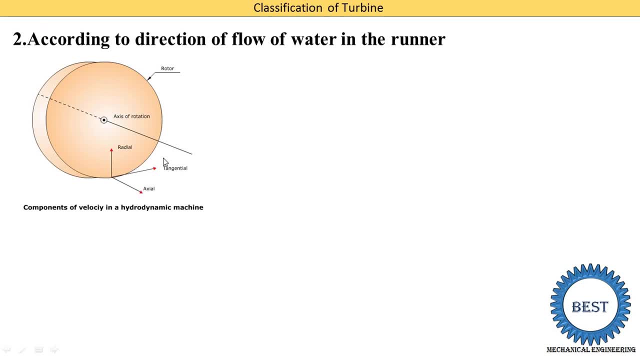 second one is the radial, third one is axial and four one is the mixed flow. now, this line we are considering, it is a sub and this circle is our runner or a rotor. okay, so tangential means the water jet is touch at the one point of this runner. that means this direction, here it is water. 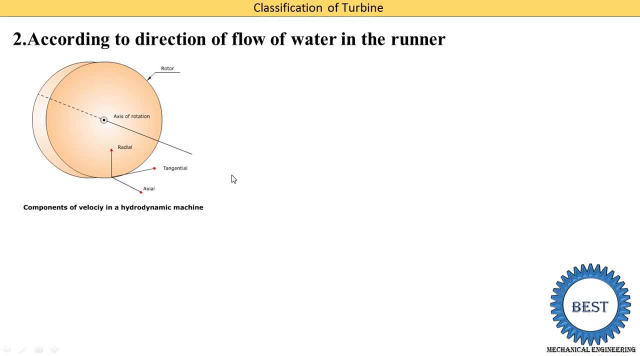 is touch to this point of the runners and exit. it is known as the tangential second. in radial direction means it is flow in the radius of the rotor or a runners. okay, so the we know that it is a center point of the runner, so we are considering it as a sub and this circle is our. 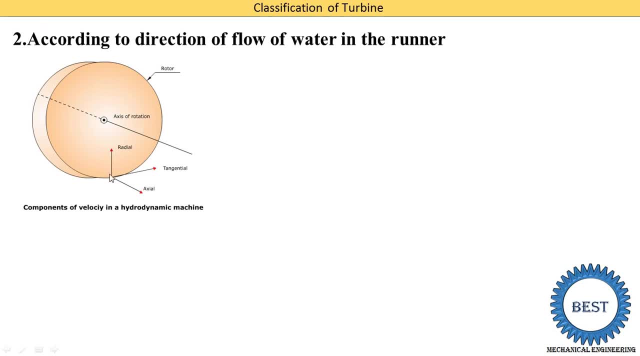 and center point to the periphery. it's known as the radius. okay, so this water is flowing in a radial direction, means: follow the radius, then it is known as the radial flow. and last one is the axial. axial means this is a shaft, it is also known as the axial, and this water 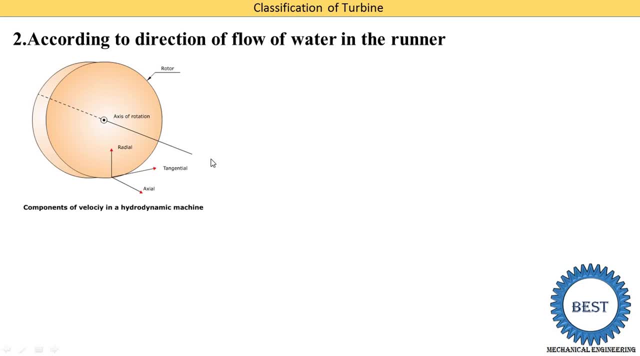 is flowing parallel to this axis, it is known as the axial flow. now we understand these in details by using these different figures. so first I explain you the tangential flow. in this tangential flow, this is the runner, this is the nozzle, and from the nozzle water. 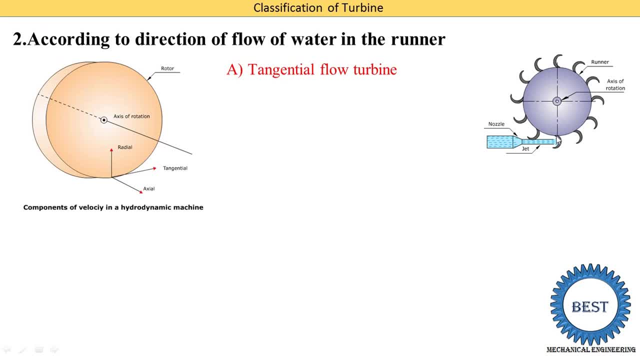 jet is coming and water jet is strike at the one point of the liner only. it is known as a tangential flow. so here the I write that water strike at the one point of the runner. it is known as the tangential flow. in a tangential flow there is a example- is pelton wheel turbine, so that 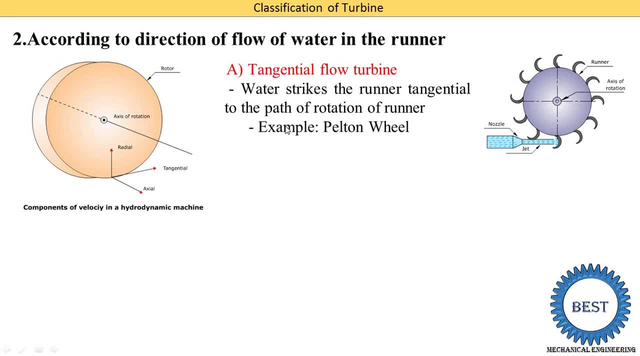 is the second point. in pelton turbine, first pelton wheel is impulse turbine and second is calton wheel is a tangential flow turbine. second one is the axial flow turbine. axial flow means water is flowing parallel to the shaft of the turbine. it is known as the axial flow. 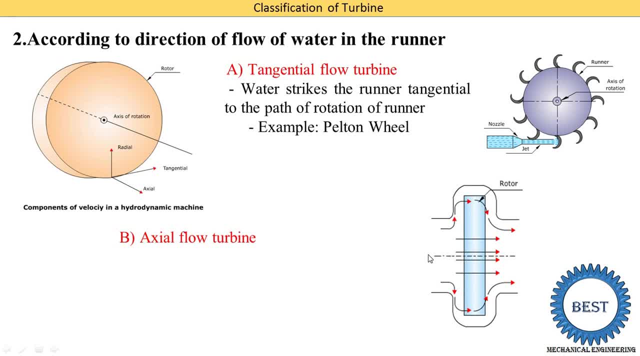 now, this is the blue part is the runner here? it is the shaft. okay, and what? this is the direction of water. so water is flowing parallel to the directions of the shaft. it is known as the axial flow. an example of this axial flow turbine is the kaplan turbine and propeller turbine. now, if you 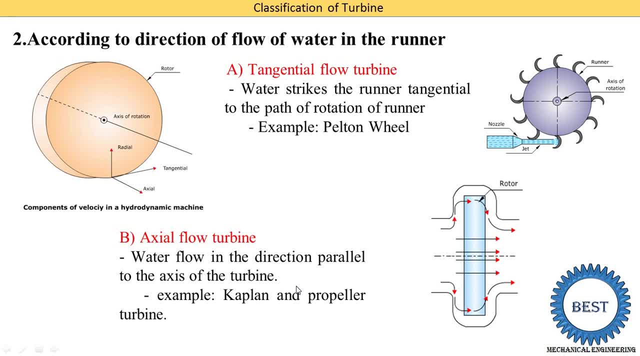 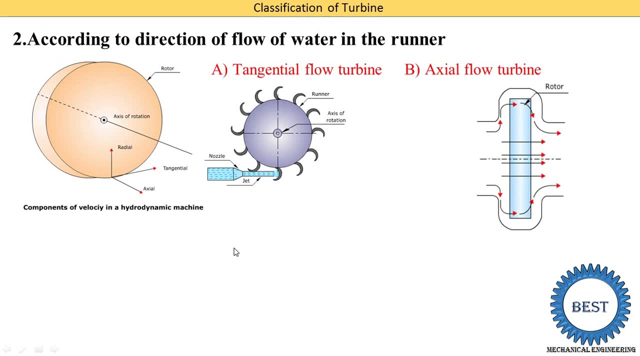 want to learn different types of turbines, then go to the playlist in which there is a hydraulic turbines and you watch the different types of the turbines and the link is also provide on this description. so the axial example is kaplan and propeller turbines. now third is the radial flow. 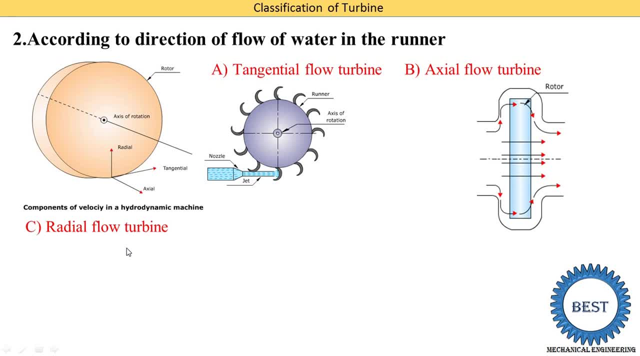 turbines. now, in radial flow turbine there is a other two classifications is there, that is, a radially inwards and radially outwards. so here i putting that the water flow in a radial direction for the runner means radius. now, in that there is a two, one is the radially in and radially outwards. so this first one is 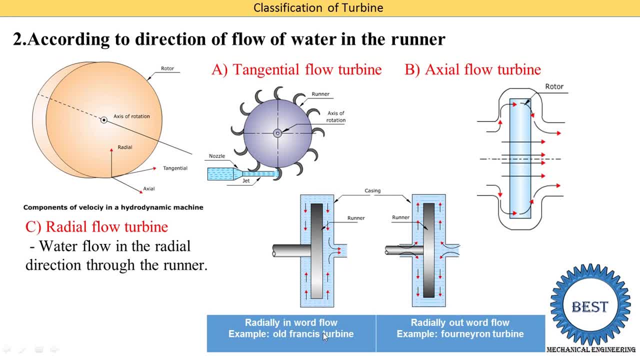 radially. inward means. name is what inward means: water is coming from outside or outer periphery and it's moving inside. that's why it is known as the inwards. so how to remember that inwards means water is coming from outside to the center of the runner. it is known as the inverse and its example is the: 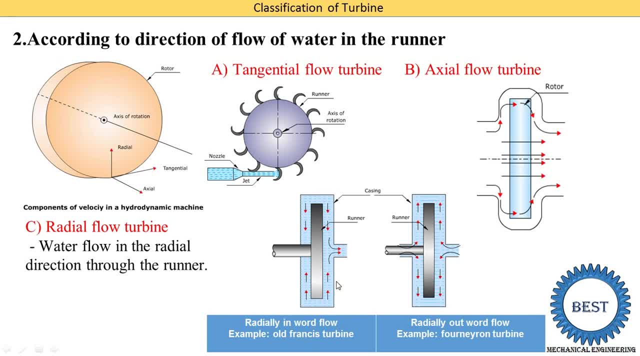 old francis turbine. so in old francis turbine that is a radially inward flow is used. now another is radially outward means in outward water is enter at the center parts and the water is flowing towards the outward directions means it is known as the radially outward flow. water flow from center. 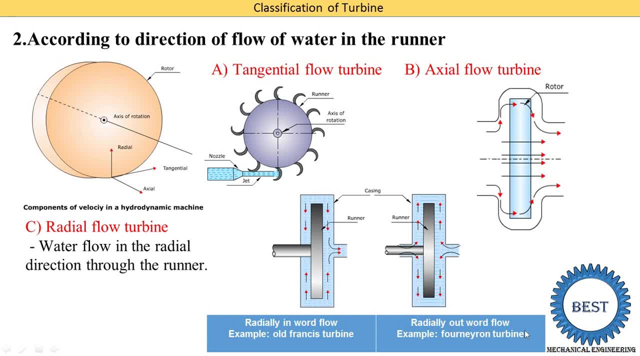 parts, to the outward parts of the water is an outward flow. so what you know, this is called radial to the outer side, then it is known as the outwards and it's example is the for Rion turbines. it's the example of the outward flow. again, i request to subscribe the channel and 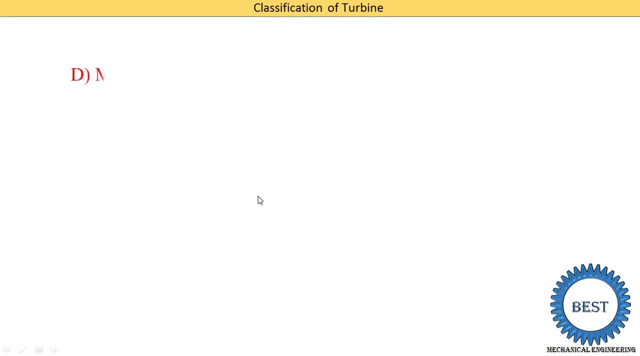 like the video. now. next point in this is the mixed flow turbine. mixed flow means the water in utter directions and water outlet is in utter directions, so here i use this figure. so this arrow is inside, means water is coming radially inwards and south is vertical. 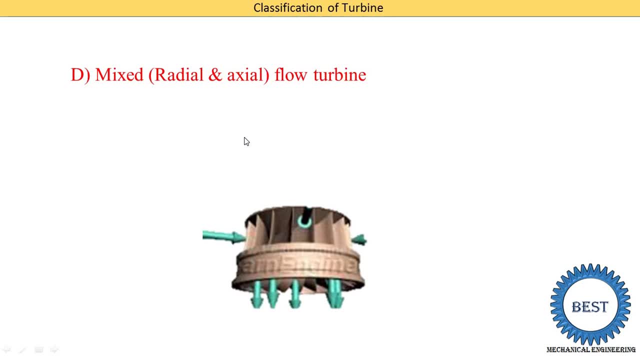 so water is outlet in axial direction. it is known as the mixed flow turbine. so water in radial directions and out in axial direction. it is known as the mixed flow turbine, and it's example is modern francis turbine. so recently the modern francis turbine is used. 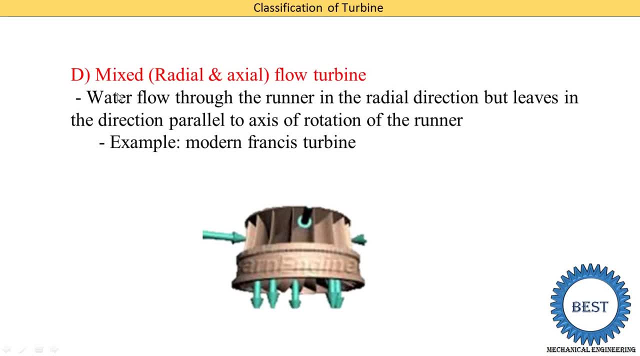 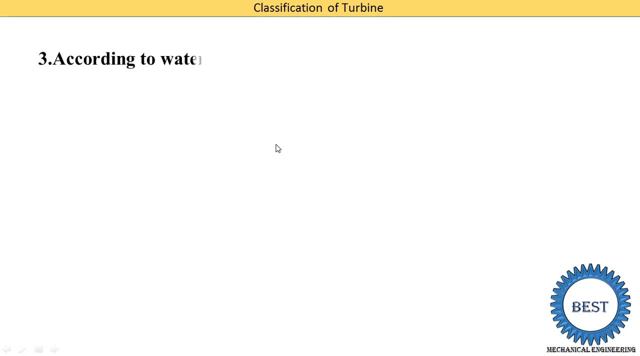 and in that the flow of the water is a mix mix means radially in and axially outwards. so recently modern francis turbine is used. old and inward and outward flow is not used right now. next classifications according to the water head and quantity of water. 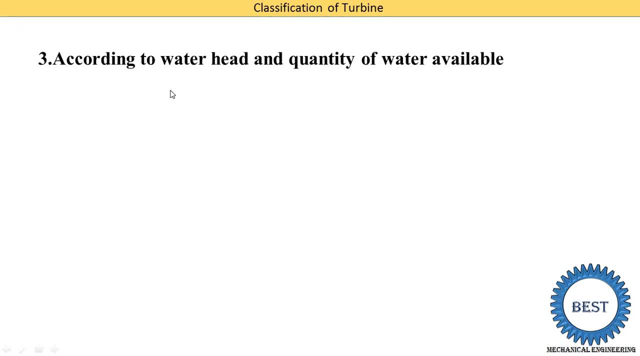 so according to the head it is classified on a three category, that is, a high head, medium head and low head. so first classification is the high head and small quantity. so with the high head that is a small quantity. if medium head, then medium quantity, low head and high quantity. that is, quantity is opposite to the head. 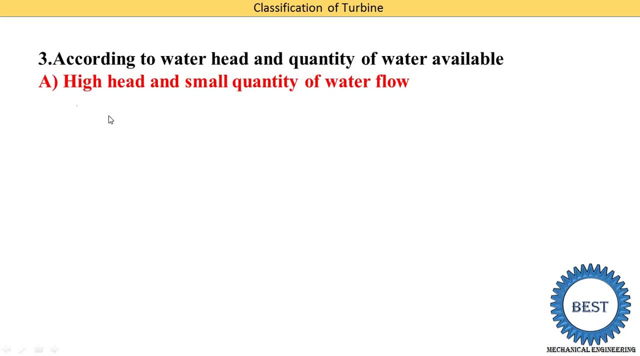 if head is high then quantity is small. now, high head means the water head is above 250m. head means what? head means water level in the reservoirs and the turbine installs means there is a difference of height between water levels and turbine. it is known as the head. 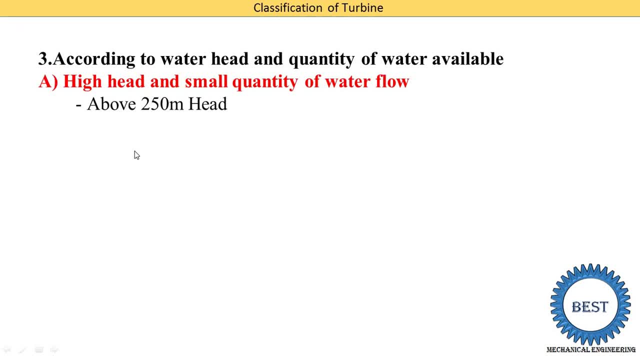 and head is greater than 250m and it is a than 250 meter and it is known as the high head turbine. and example of high head turbine is the Peltonville turbines. okay, so in a hydro power plant, if the water head is available greater than 250 meters, then it is known as the Peltonville turbines and Peltonville is. 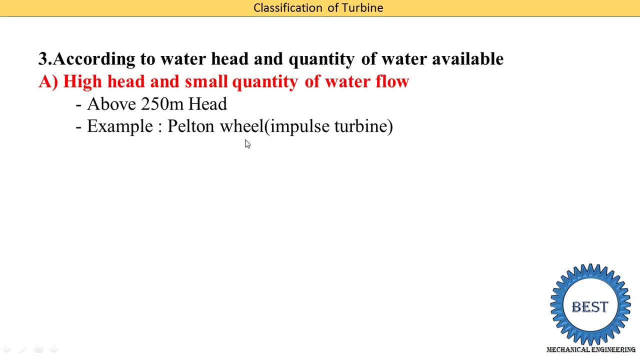 also impulse turbine. so we learned a three point in Peltonville turbine: first, impulse, second is tangential flow and third one is the high head and fourth is the small quantity of water. second one is the medium head and medium quantity. for that head limit is 60. 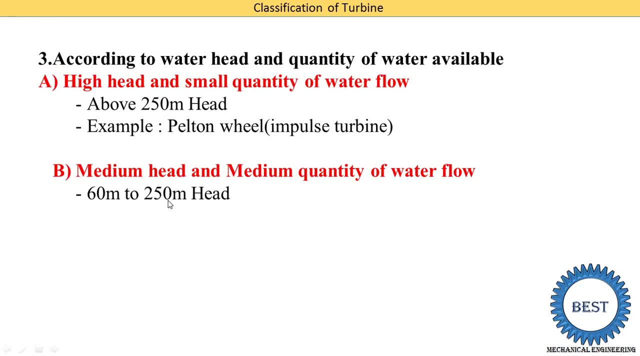 meter to 250 meter. head means water level in reservoir and turbine installs. that difference of height is 60 to 250 meter. then the we use the Francis turbine because example of this is a modern Francis turbine and it is known as the medium head and medium quantity. next, 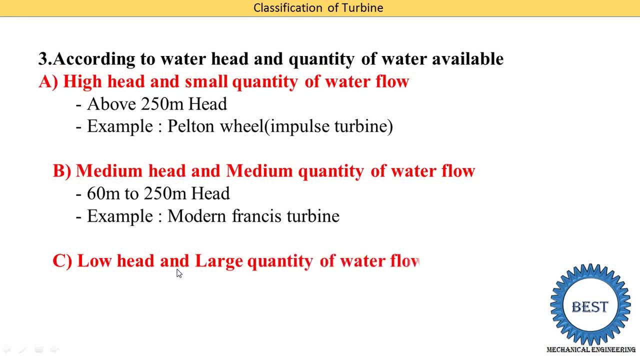 point is the low head And the larger quantity of water. low head means head below 60 meter, it is known as the low head turbine and the quantity of the water is large. and example of this low head is the Kaplan turbines and propeller turbines. so in Kaplan turbines again we learned the four. 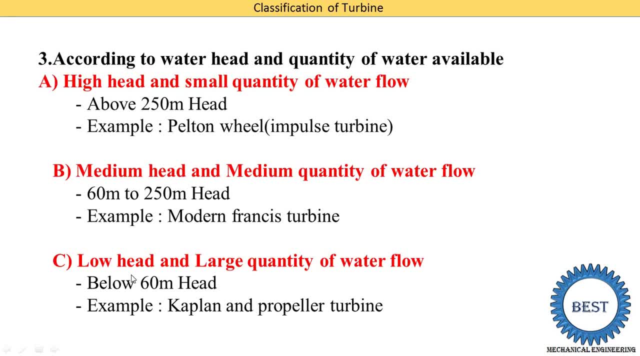 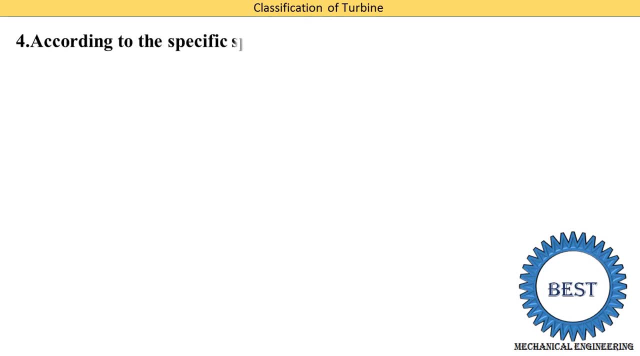 point. first one is reaction turbines: flow is axial and the low head turbines and the larger quantity. Now last classifications. after that classification, I Will give you the summary and three for remembering that. so according to the specific sphere, that is, the low specific sphere, medium specific sphere and high specific sphere, if you want. 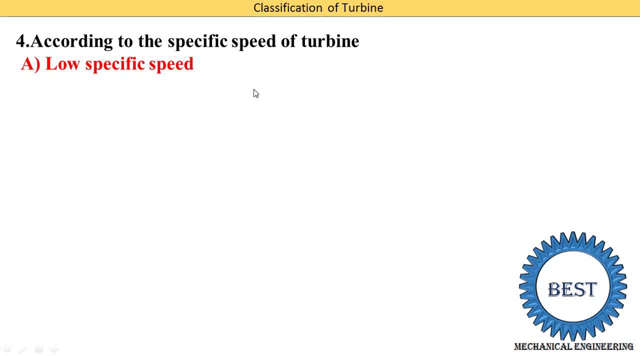 to know the what is the specific sphere? then watch the my video on the specific sphere. that link is provide on description as well as also in the playlist. Low specific sphere means specific sphere is less than 60 and it is known as the specific sphere. now, the rpm, that is, a revolutions per minute of turbine, is different and specific. 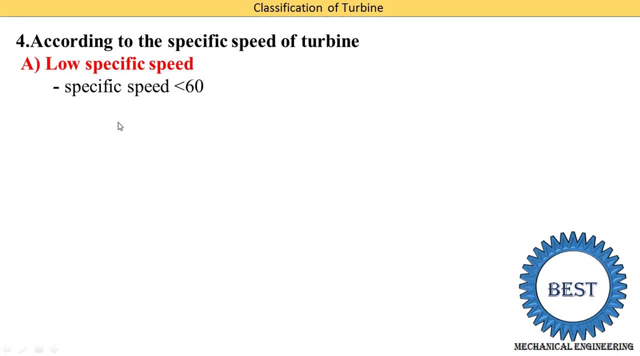 sphere is different. it's not the same. okay, so it is a different thing. And it's example of the low specific sphere is the Elton will turbine. So we learn five points and I summarize at the last of the video: medium specific sphere means specific sphere is in between the 60 to 400, means medium is 60 to 400 and it's. 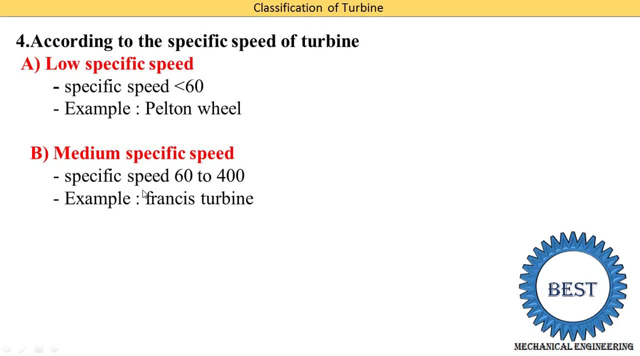 example is the Francis turbine. So here you see that in the Francis turbine All Everything is coming to medium Okay. So these are the simplest take trick to. in Francis turbine everything is the medium okay. and the last one is the high specific sphere. high specific speed means specific speed is. 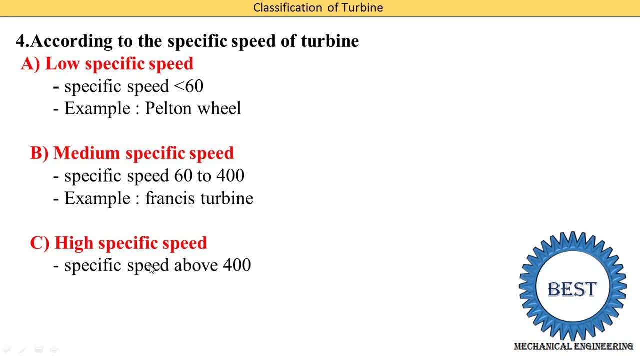 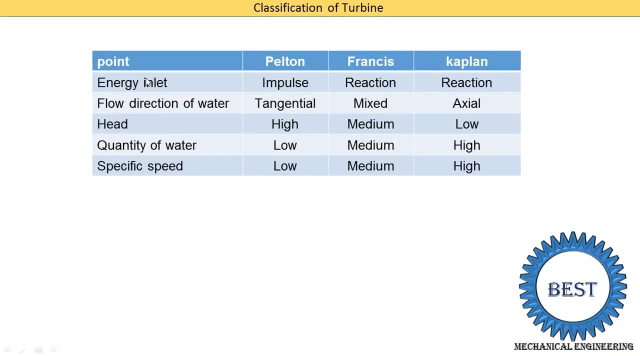 greater than 400 over 400, and his example is the Kaplan turbine and propeller turbines. now here I. so it is trick, that is a point. first classification: we learn according to energy inlet. Here This is a different turbine, first column Pelton, second Francis, third one is Kaplan, as a only. 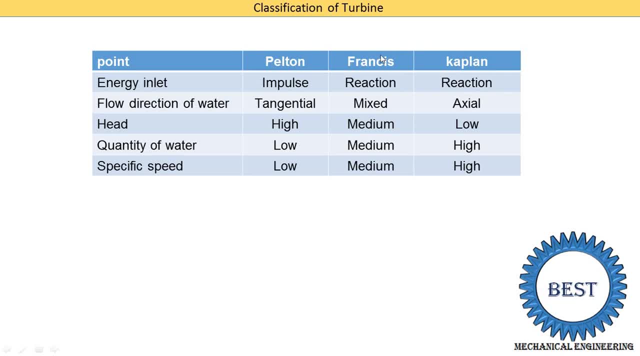 impulse turbine, that is a Pelton will turbine. another two is the reaction turbine, Francis and Kaplan. second point is the flow direction of water. it is a tangential flow in Pelton turbine mix, in modern Francis turbine and in a Kaplan. that is a axial flow. okay now.